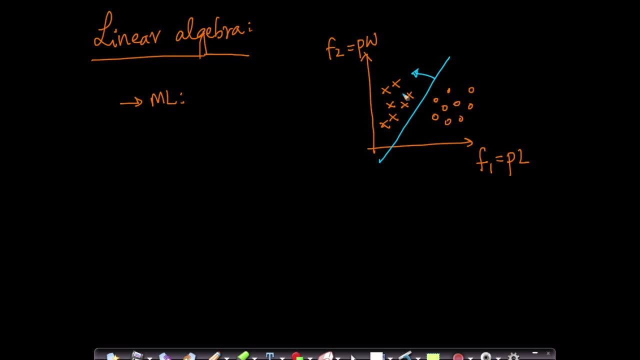 everything on one side of the line belongs to one class of flowers. Everything on this side belongs to another class of flowers. right? This we could do it in 2D. Imagine if I had to do the same thing in 3D. what would I do? Imagine if I have three features. right, Feature 1, let's say: 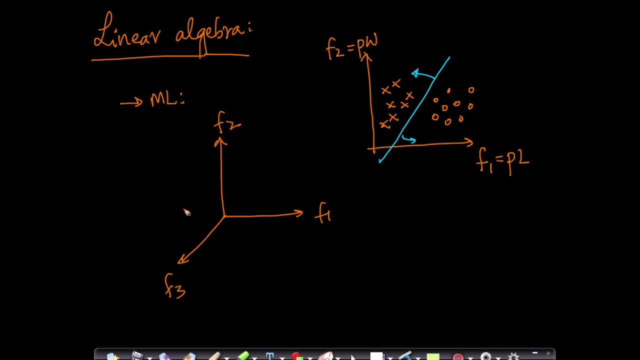 feature 2 and feature 3, right. And if my points were like this, right In my three-dimensional space, right, I could again draw a plane like this. I could draw a plane like this and say: everything on this side of the plane belongs to one class of. 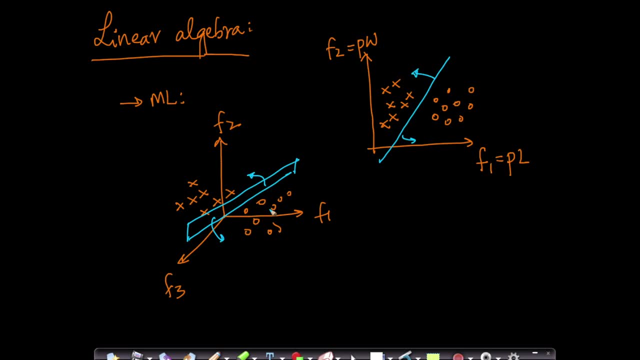 flowers. Everything on this side of the plane belongs to another class of flowers. Now, in 1D, we have a line to separate. In 2D, we have a plane. What about 4D? What about 5D? What about 10D? What? 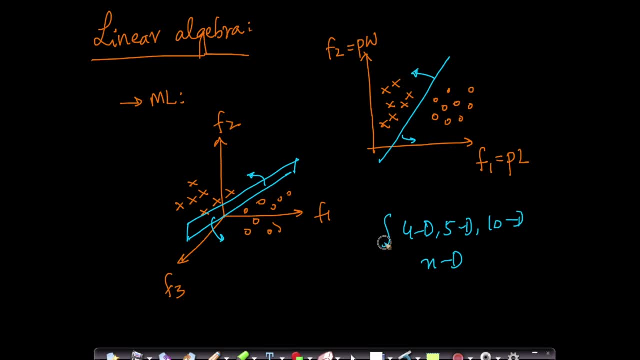 about any dimensional space. What happens? How do we understand the equivalence? So here you can think of a line as a linear surface that is separating a line from a plane. So here you can see the line separating one class of points in another class, same with a plane. right, It's also. 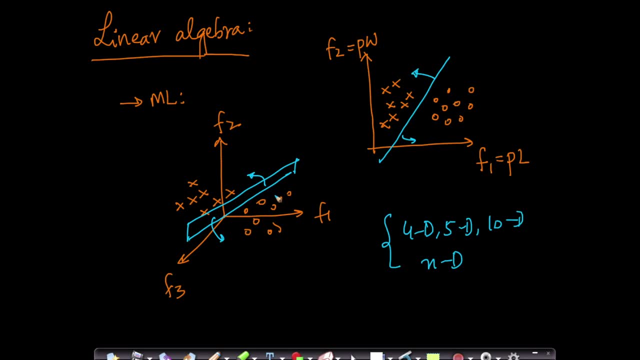 a linear surface which is separating one class of points from other class of points in a 3D space. Now, whatever we have learned in 1D, 2D and 3D, how do we generalize it to higher dimensional spaces? Of course we can't visualize the data in 4D, 5D, 10D or ND. Linear Algebra is the brilliant. 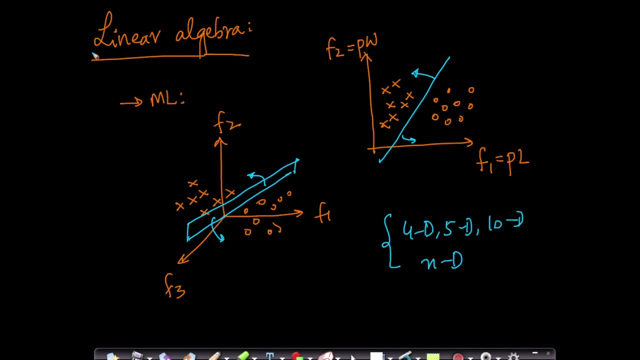 mathematical tool that we have at our disposal to help us take our learnings, our understanding, intuition, from 2d and 3d to higher dimensional spaces. we will see. we will see that your line, your plane, all these things are connected through beautiful and very simple and elegant mathematics. 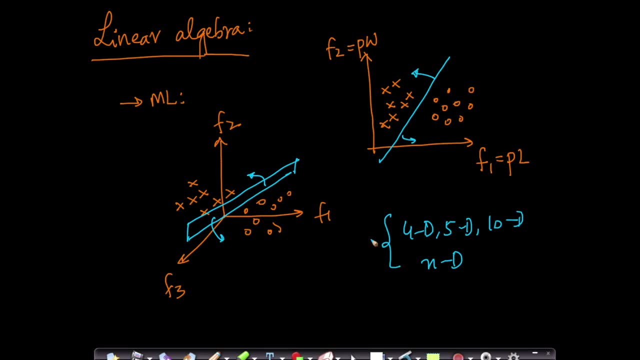 linear algebra provides us those mathematical tools to help us operate in higher dimensional spaces. because in machine learning, if i have 10 features i'm operating in a 10 dimensional space. right, if i have thousand features, i'm operating in a thousand dimensional space. but of course we 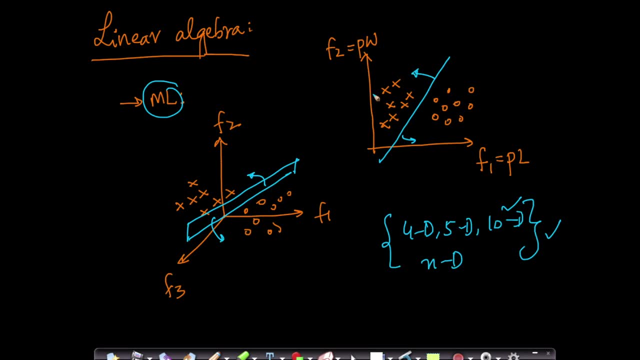 can't visualize anything more than four or five d right, and hence linear algebra provides us with the mathematical tools that we need to simplify and to generalize our learnings that we learn from 2d and 3d.